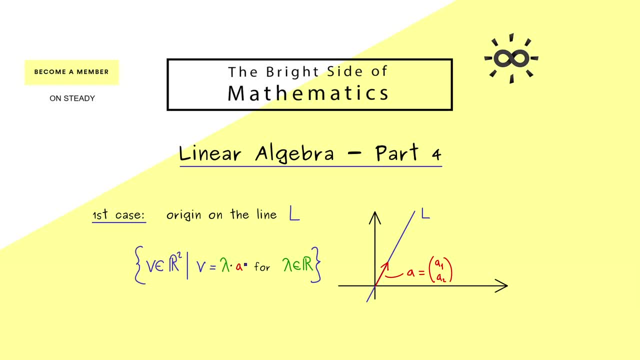 v that fulfill that. they are given in the form lambda times a, And then we are finished. the line L is described with this set. So you see, we only have to put in one vector for the direction. However, another possibility would be to take a. 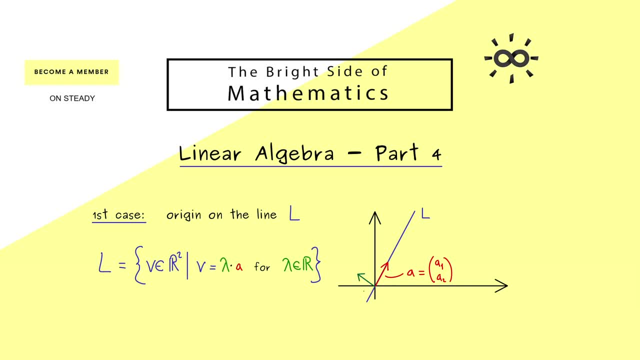 vector that is orthogonal to a. So you already know we need the inner product to talk about orthogonality. So for the moment, let's call this new vector here simply n. And now what you should see is this: n is perpendicular to the whole. 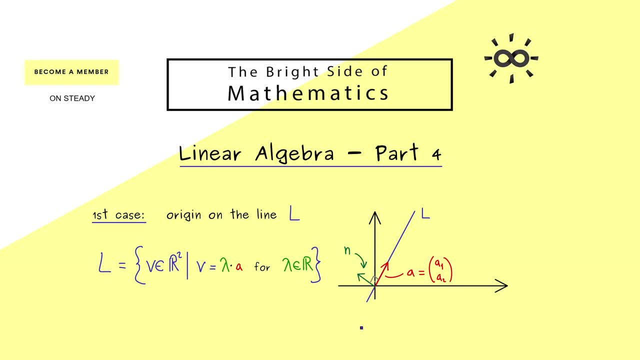 line L. Hence this is an alternative description for the line L, So we only need a so called normal vector n to define this set You More precisely, we would say: this is the set of all vectors v, with the property that the inner product of n with v is exactly 0.. 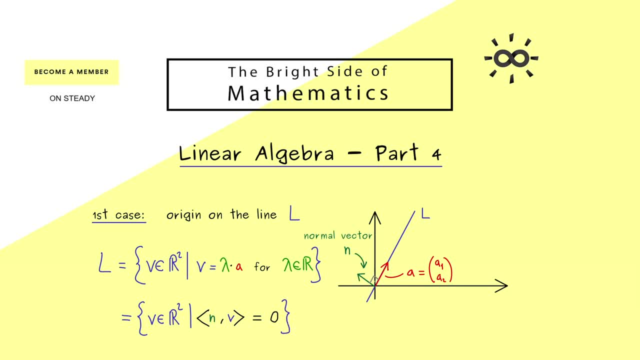 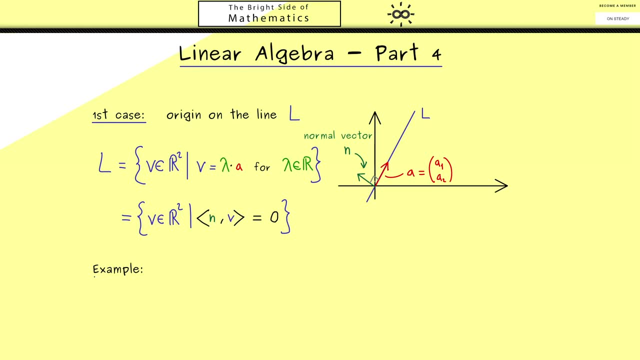 Because this is what orthogonal means. Ok, there, it might be helpful to look at an example. So we just take a normal vector, n, and then we define the line l, For example. let's take this vector here, which should be 3 minus 1.. 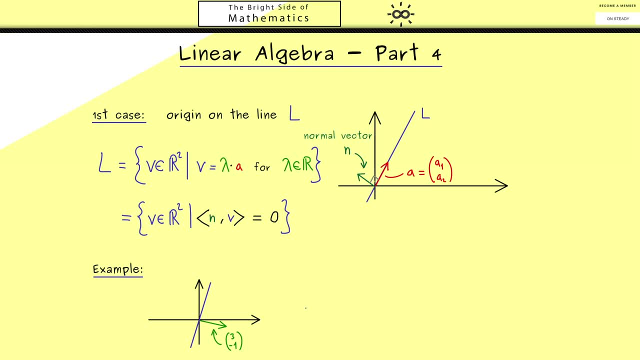 Hence, then, the line l should look like this. Now for the set description. we already know what to do. We write down l as v in R2, with the property that 3 minus 1 with v in the inner product is equal to 0.. 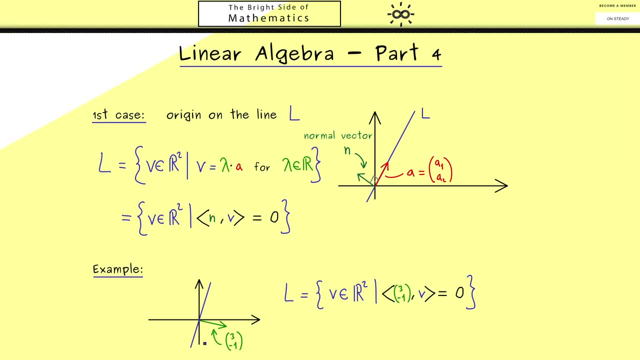 Ok, so maybe you are used to the variables x and y for the coordinates. Therefore, instead of v, we could also write x, y, And then we can just simplify the inner product on the right hand side. So don't forget, this is the standard inner product. so we multiply 3 with x and minus 1 with y, and then add them. 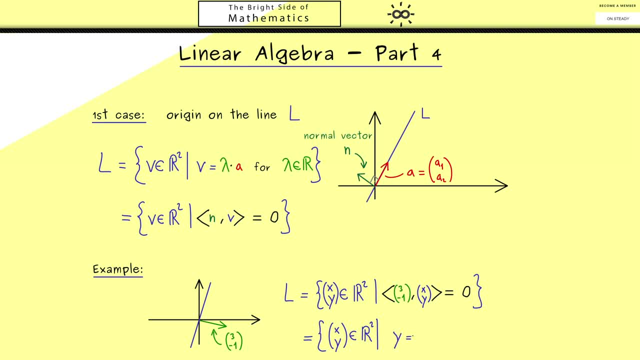 Hence we can write the equation as: y is equal to 3x. And there you see, this is how you would describe this line as the graph of a function. So i would say everything is fine. So i would say everything is fine. 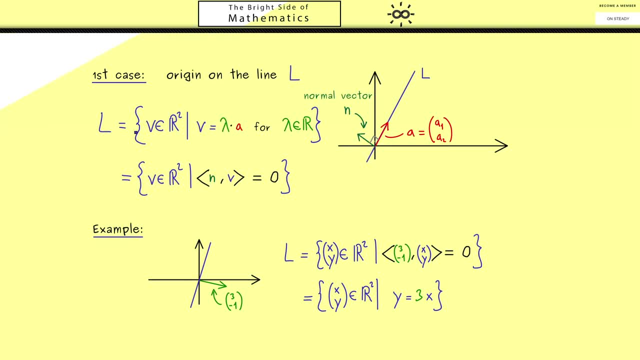 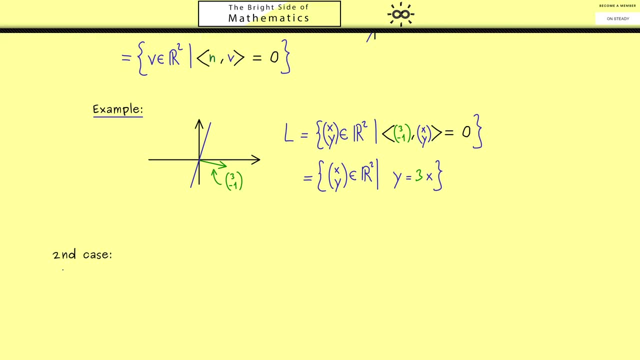 So i would say everything fits nicely and therefore we are ready for the second case. This is the general case where the line does not have to go through the origin. Also there we should start with a visualization. So here we have the plane again and maybe one line here. 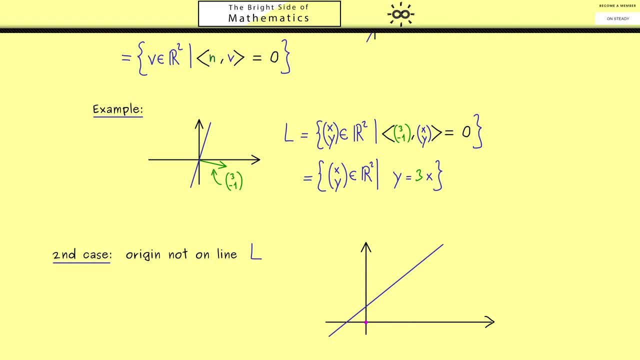 And now you could say: this line is translated from the origin to this point here, Then this translation is given by a vector p, Then this translation is given by a vector p, Then this translation is given by a vector p. This shouldn't be a problem for us, because we know the vector addition. 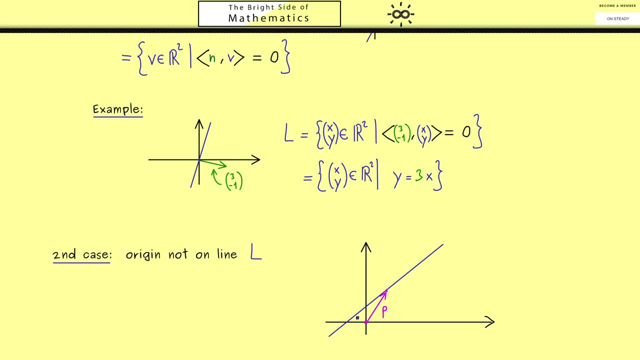 More concretely this means when we take another point here on the line and describe this with a vector v, Then we know, when we form the vector addition of minus p, plus v, we have a vector in the direction of the line. 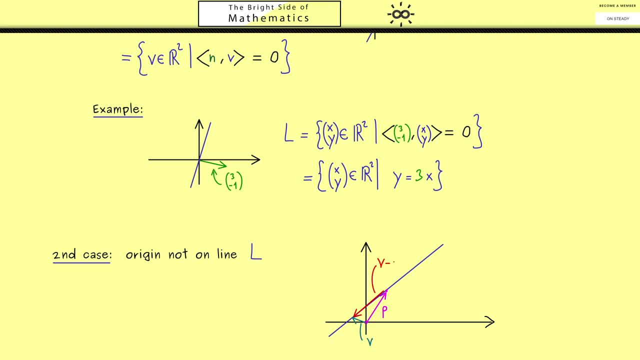 So don't forget this here represents the vector v minus p And you see, no matter which point v we choose on the line, this vector will always be in the direction of the line. This vector always shows in the direction of the line l. 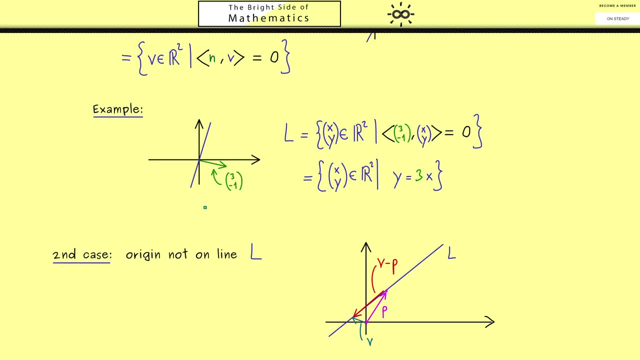 And therefore we can do the same thing as before and use a normal vector. Then this vector v minus p is always orthogonal to the normal vector n. Ok, then let's write this down: l is the set of all vectors v in R2.. 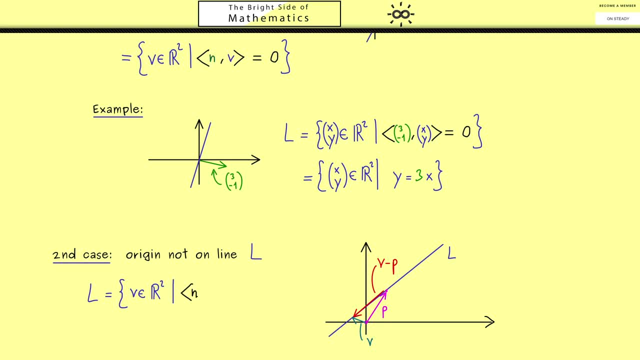 With the property that the inner product of n with v minus p is 0.. So you should see, the only thing we have to put in here is a normal vector n and a vector p, And then these two vectors describe the whole line. 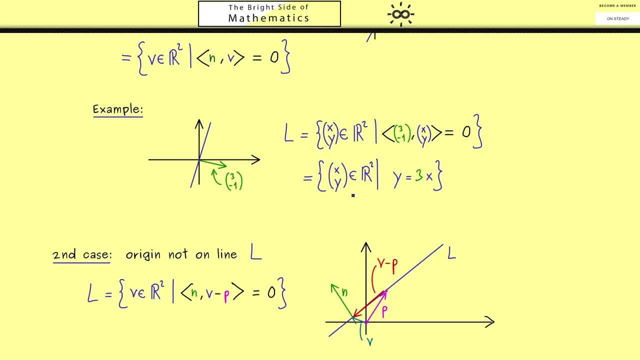 However, as before, we can simplify this even more and maybe we use x and y again. So we have the set of all points x and y in R2.. And then, when we simplify the inner product, we have n1 times x plus n2 times y is equal to a constant we can call: 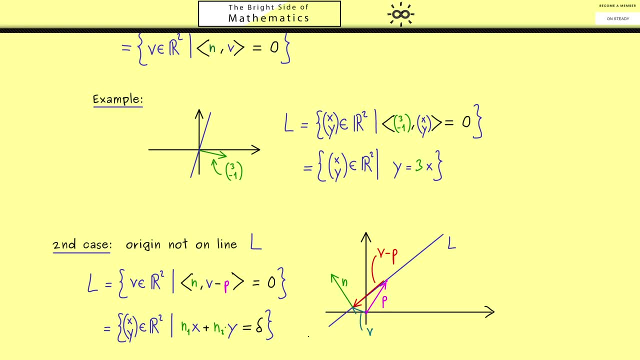 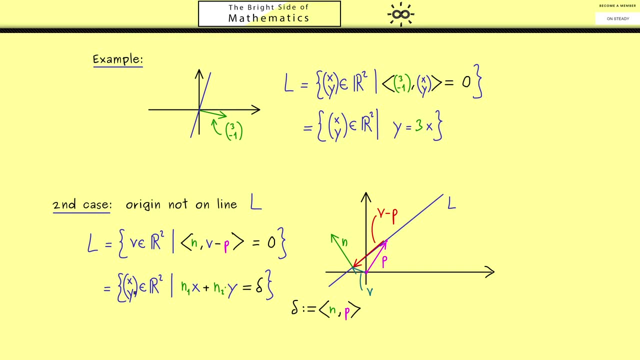 delta. And now this constant delta is just the inner product n with p. We say it's a constant because it does not depend on the numbers x and y, it's just a number that comes from the line l. So in summary, you should see, with only three numbers, and 1 and 2, and delta.